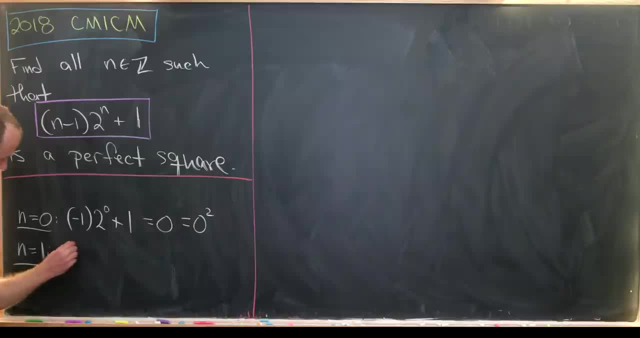 to n equals 1.. Well, n equals 1 is 0. So we get 0 plus 1, which is 1.. But that's clearly 1 squared, So that works out as well. Then now let's look at n. 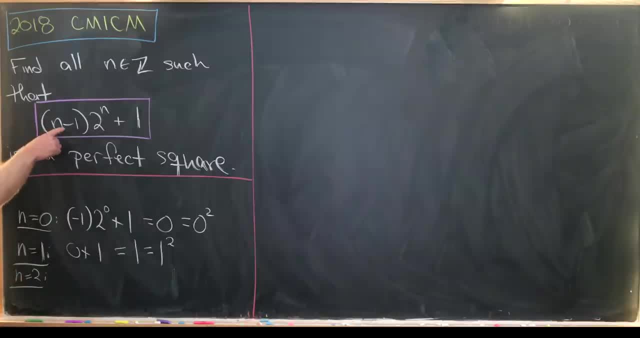 equals 2.. So n equals 2.. We get 2 minus 1, which is 1.. 2 squared plus 1.. So 2 squared plus 1 is 5.. So that does not give us a solution. So just to reiterate, we do have a solution here and here. 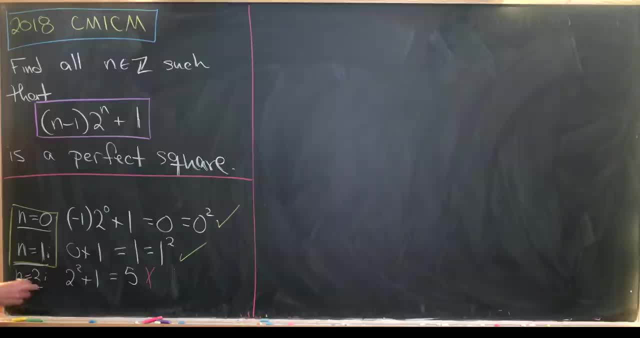 So these two numbers are good, But this number right here- n equals 2, is not good. I'll let you check n equal 3 on your own, but you will not get a solution in that case. So let's go to. 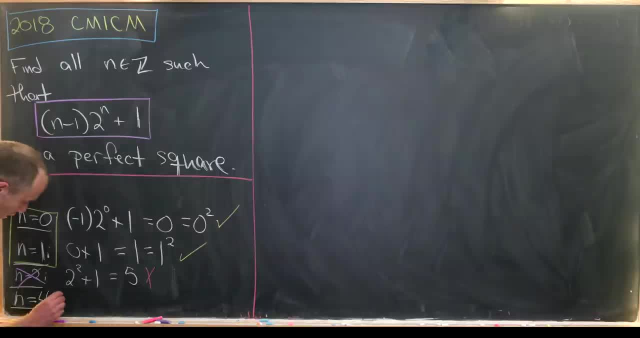 n equals 4.. So in that case we get 4 minus 1, which is 3 times 2, to the 4,, which is 16 plus 1.. That gives us the number 49,, which is clearly equal to 7 squared. So we've got another solution. 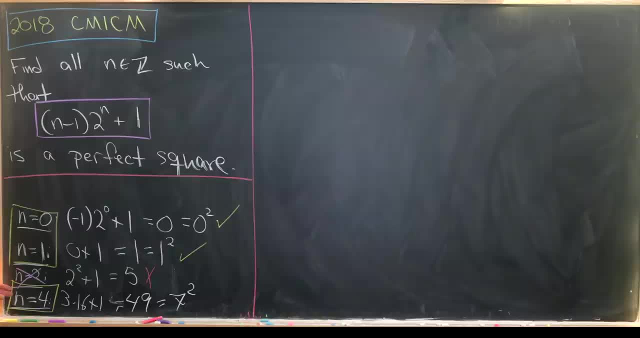 in this case when n equals 4.. Then it turns out there are no solutions after that, which we'll get to showing eventually. But before we do that, let's notice that we've got all integers here- positive integers or all non-negative integers. So that means we need to work backwards as well. 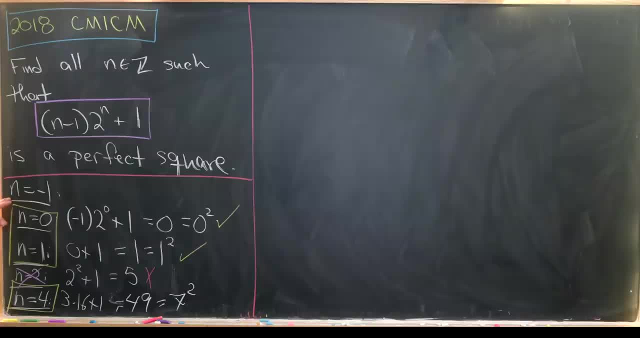 So let's look at the case when n equals minus 1.. So that's going to give us negative 2 times 2 to the minus 1 plus 1.. 2 to the minus 1 is a half times negative. 2 is negative 1 plus 1. 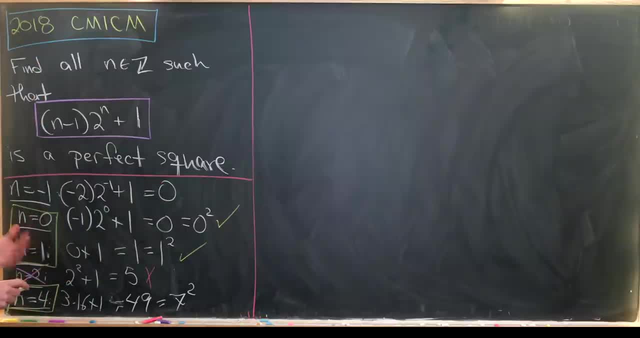 equals 0. So we get, this is 0 as well, but 0 is clearly 0 squared, So that n equals negative 1 gives us a solution. So so far we've got four solutions. Now what we'd like to prove is that: 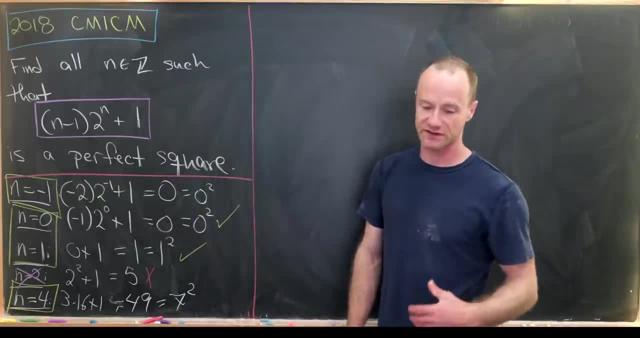 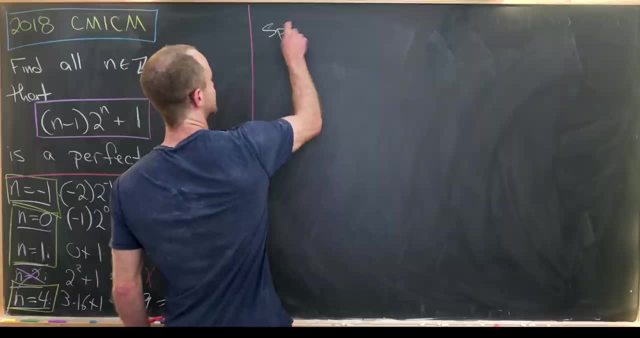 there are no more solutions up that way. So for n equals negative 2, negative 3, so on and so forth. So let's maybe do that. So first let's suppose that n is less than or equal to negative 2.. 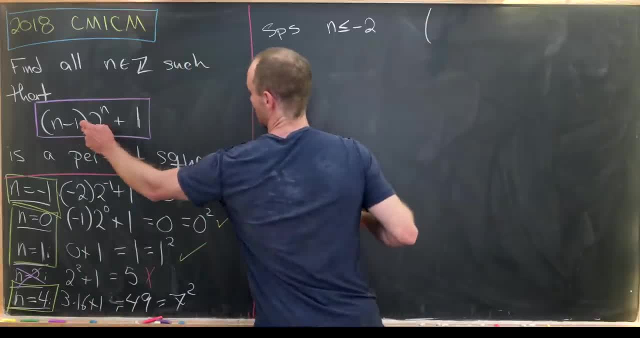 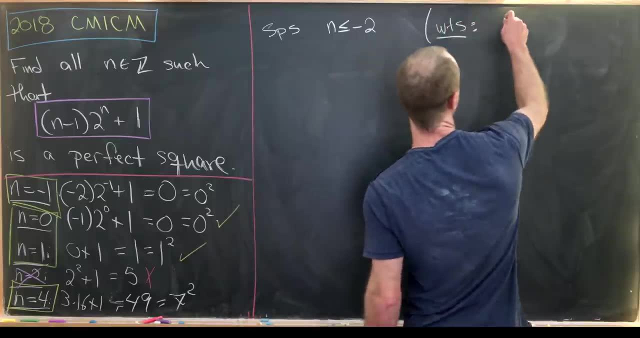 So the issue we want to build will be that this n minus 1 times 2 to the n is not an integer. So let's point that out here. We want to show that n minus 1 times 2 to the n is not an integer. 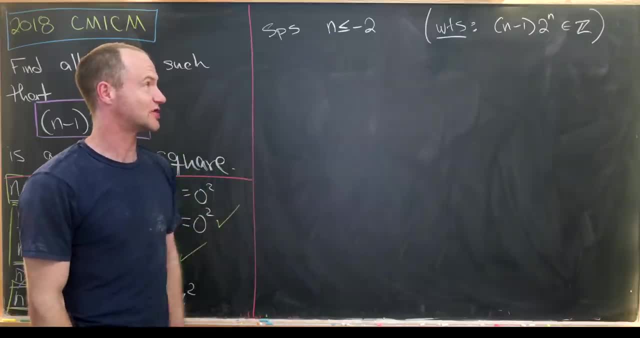 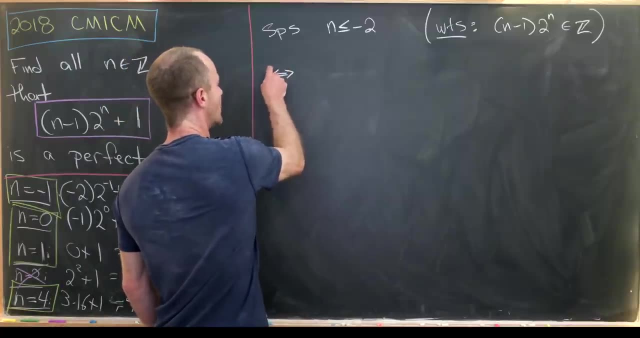 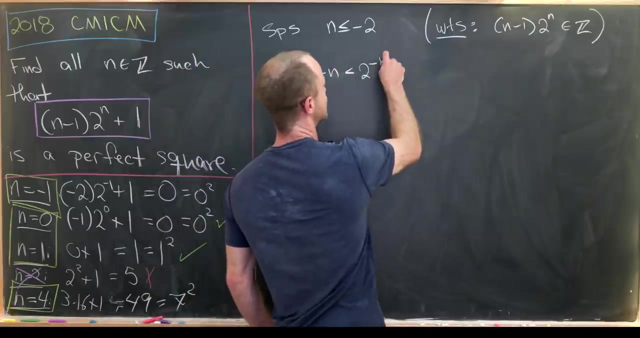 Okay, again, that's built off of this kind of assumption that n is less than or equal to negative 2.. But next up, let's note that that's equivalent to showing that 1 minus n is less than 2 to the minus n. 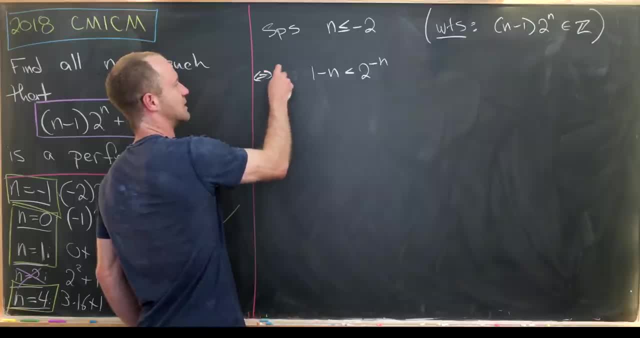 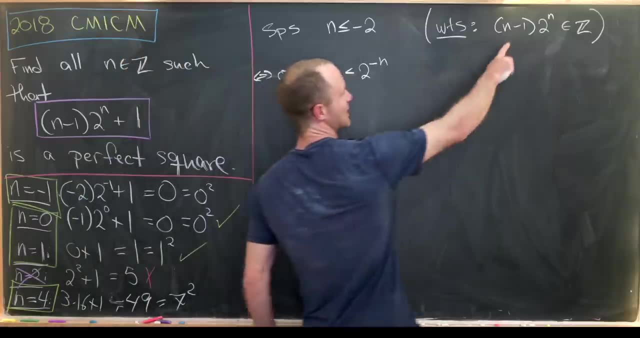 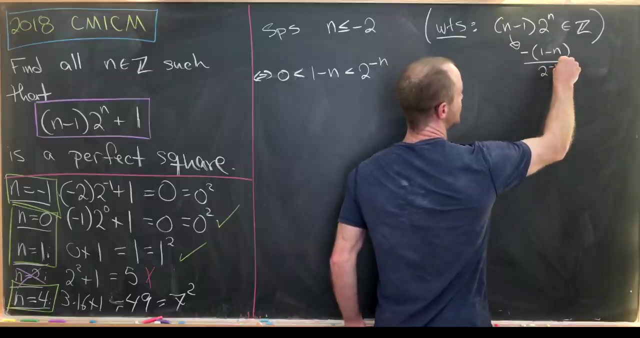 And that puts everything kind of into positive numbers here. So I can put 0 over here on this side. So notice, if 1 minus n is less than 2 to the n, then you can think about this as being like a fraction of negative 1 minus n over 2 to the minus n. But if that numerator is smaller than 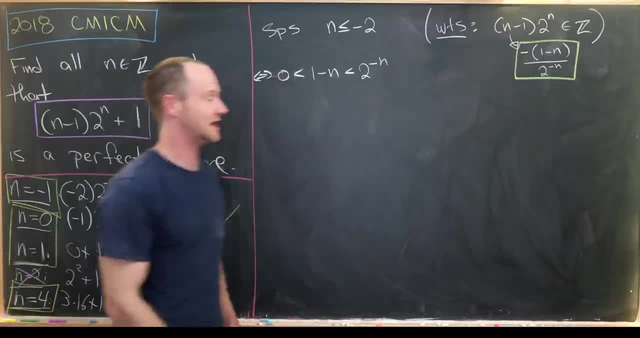 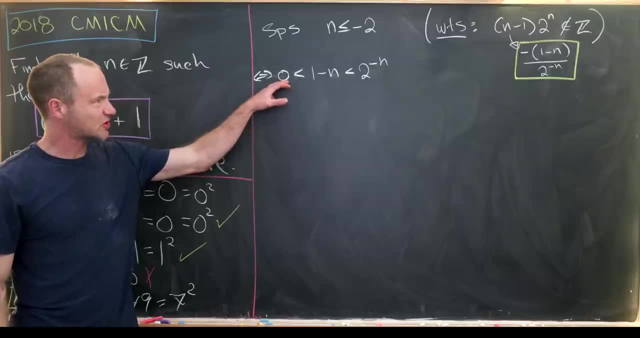 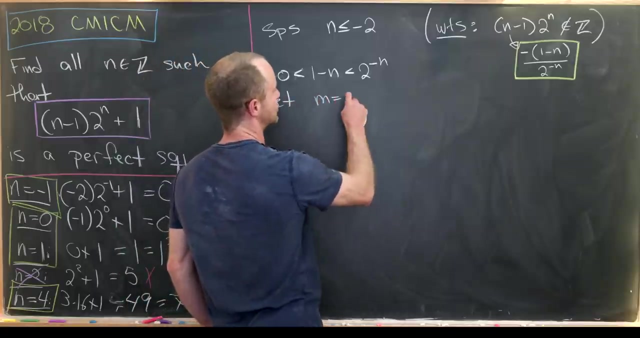 the denominator, then that thing is most definitely not an integer. I think I said not an integer, but I forgot to put my little Cross there. Okay, but it's a little bit tricky to deal with these minus signs everywhere. So let's make a change of variables. So let's set m equal to negative n, And then that means that m 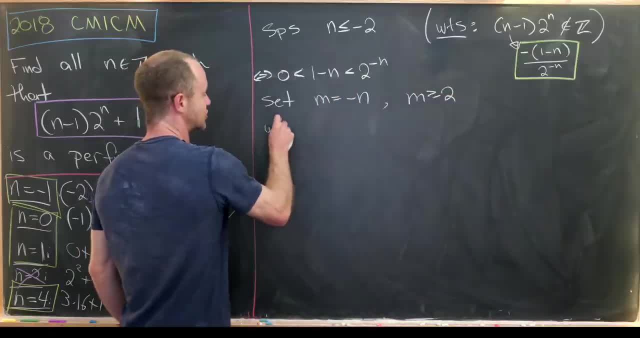 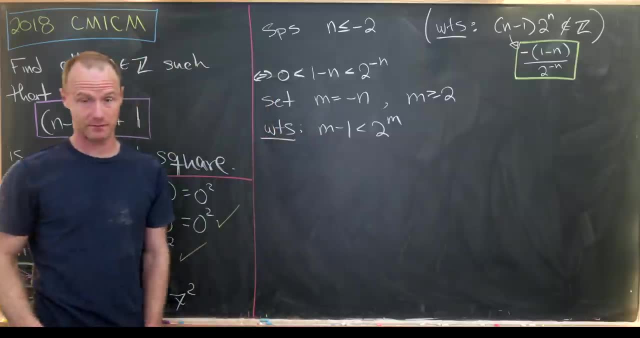 is bigger than or equal to 2.. And what we'd like to show is now that m minus 1 is less than 2 to the n. But now it's looking like something pretty familiar. We've got like a polynomial on the left. 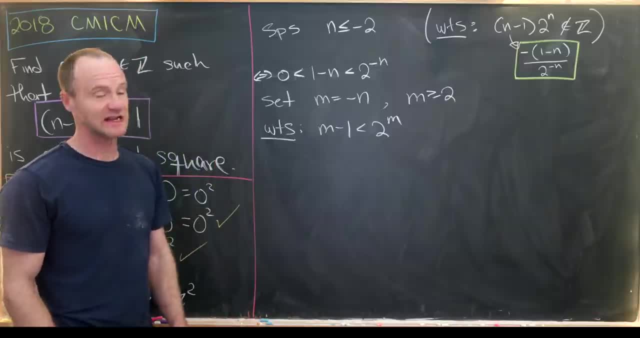 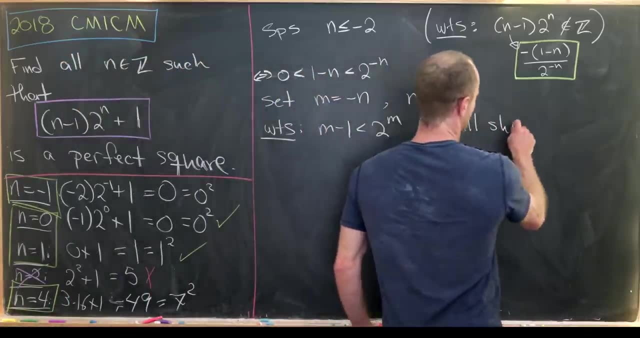 hand side and an exponential on the right hand side, And then we've got a polynomial on the right hand side. Obviously, the exponential will always win out. So what we will show instead. so we will show is that m is less than 2 to the n for all m bigger than or equal to 2.. 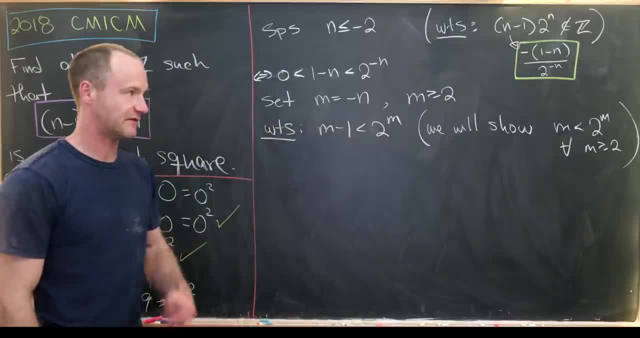 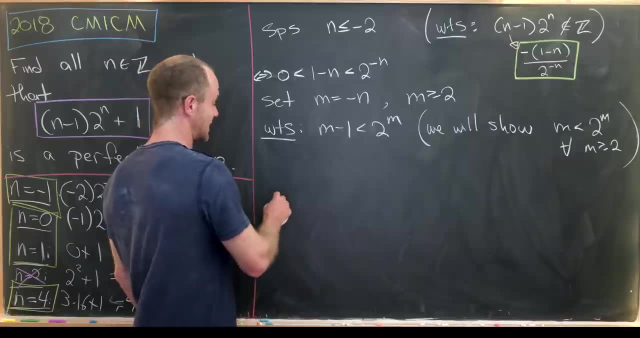 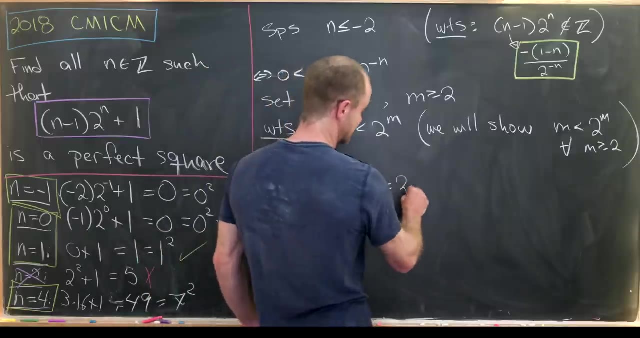 Then m minus 1 is clearly to the left of that And we can do that by induction or by like a bunch of other ways if you want to. So maybe we could do that by induction. So our base case that will be like the m equals 2 case in this case And notice that 2 is most definitely less. 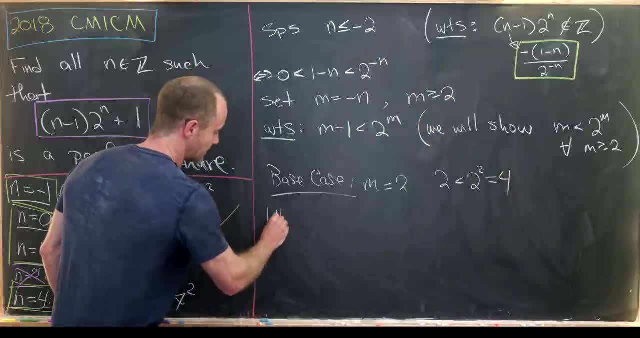 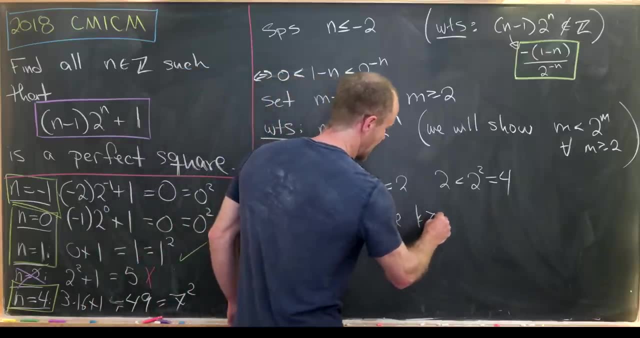 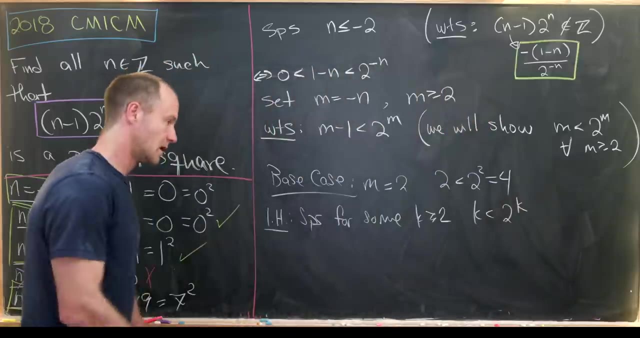 than 2 to the 2, because that's equal to 4.. And then we can make an induction hypothesis. Let's say we suppose for some k bigger than or equal to 2, we know k is less than 2 to the k. Okay, 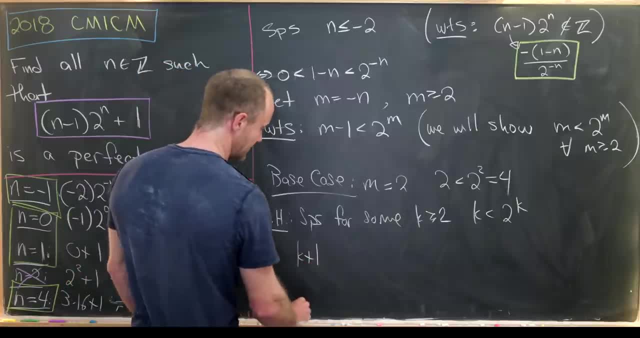 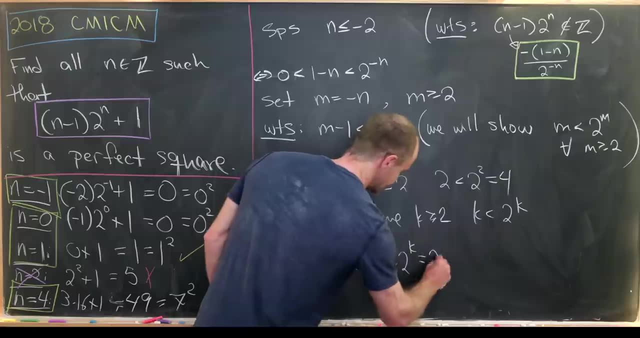 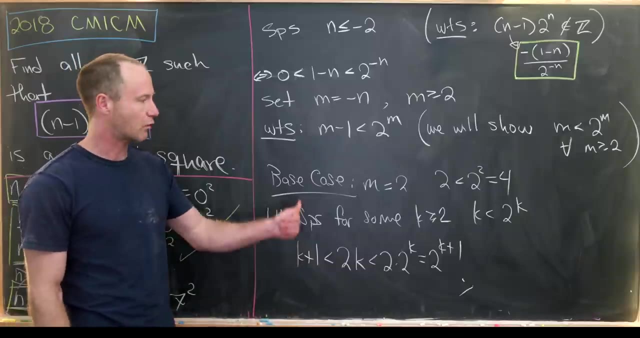 but then note that k plus 1 is less than 2 times k, which is less than 2 times 2 to the k, which is equal to 2 to the k plus 1, which is exactly what we needed to do to finish this thing off. Okay, so now let's work back up. 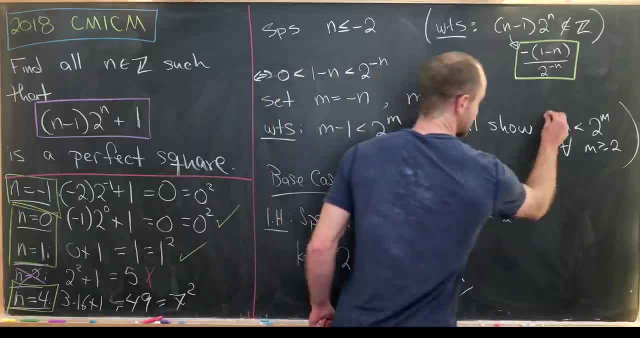 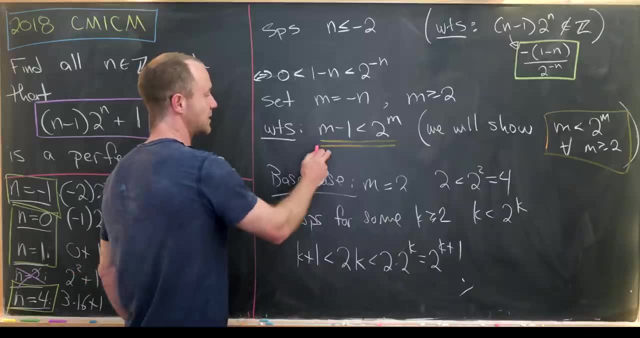 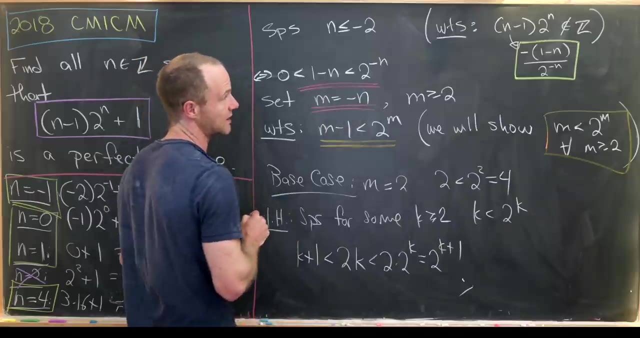 to the top. So we've just proven this inequality and that inequality implies this inequality right here. but then, via the change of variables, m is equal to minus n. that establishes this inequality, which means that this guy right here is not an integer, but if that guy right there is not an. 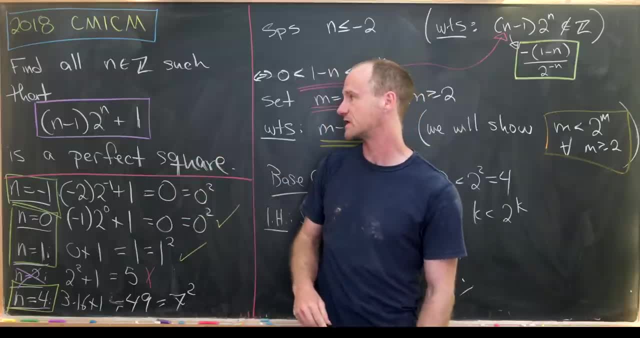 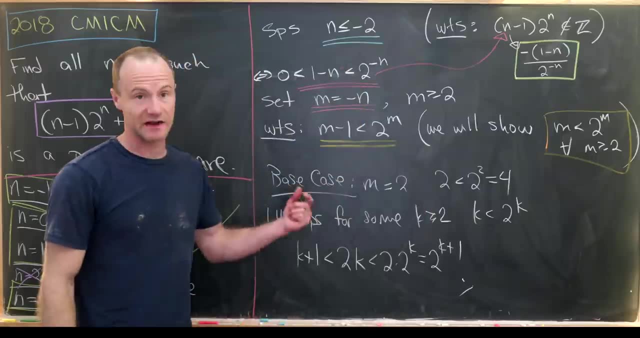 integer, then we cannot talk about this object as being a perfect square. Okay, so that clears up everything for the cases when n is less than or equal to negative 2.. Now we'll work on the cases when n is bigger than or equal to 5.. 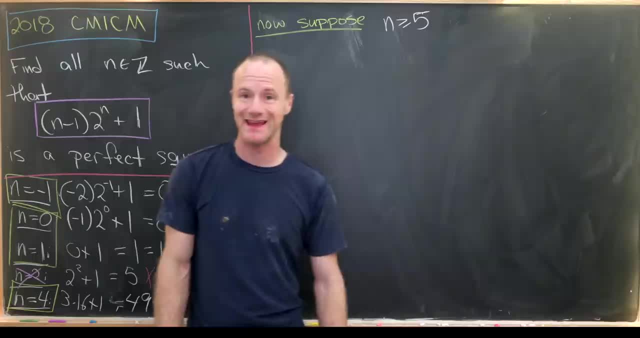 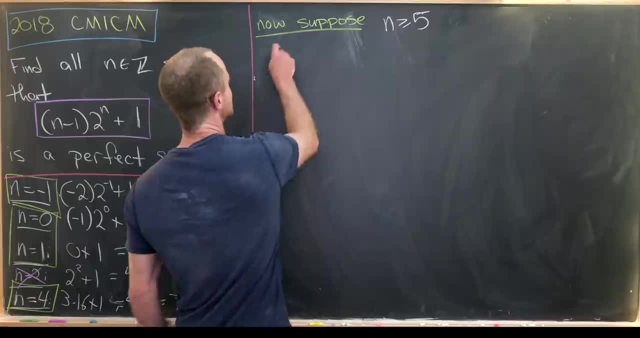 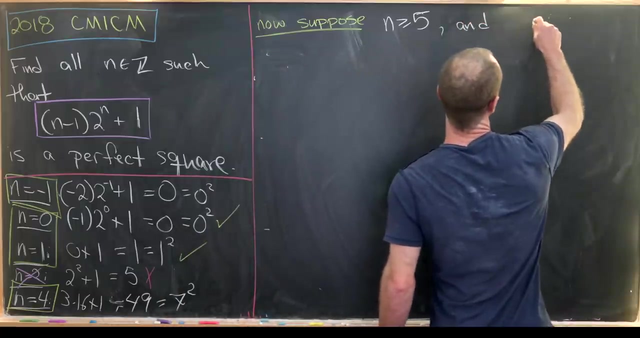 So all we're left to show is that there are no more solutions when n is bigger than or equal to 5, and that means these four solutions over here are the only ones that we have. Okay, so let's suppose that n is bigger than or equal to 5 and we have some integer, which I'll call k. We can. 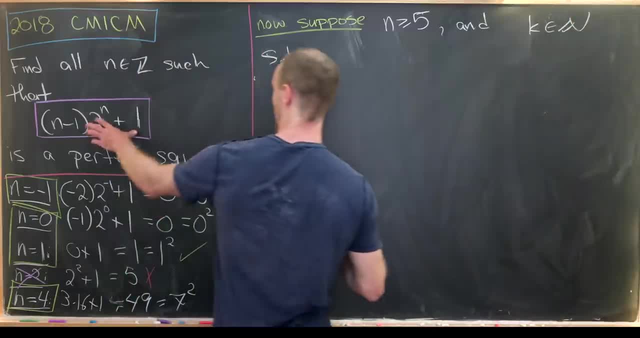 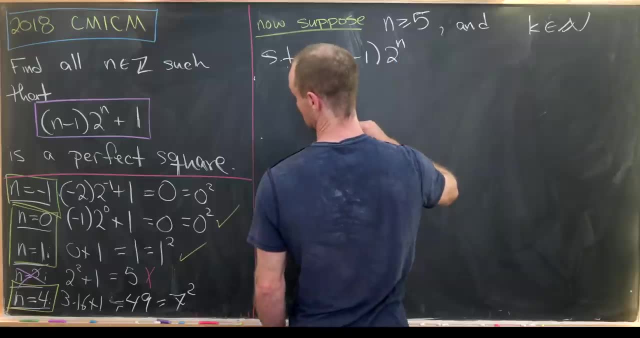 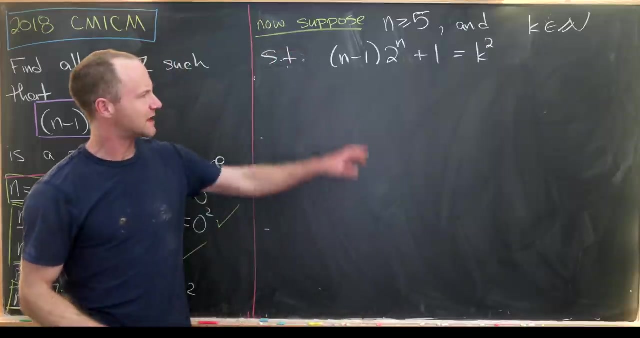 actually take it to be a natural number, such that our expression is equal to k squared. So we have n minus 1 times 2 to the n plus 1 is equal to k squared. Okay, but now let's note that the left hand side is most. 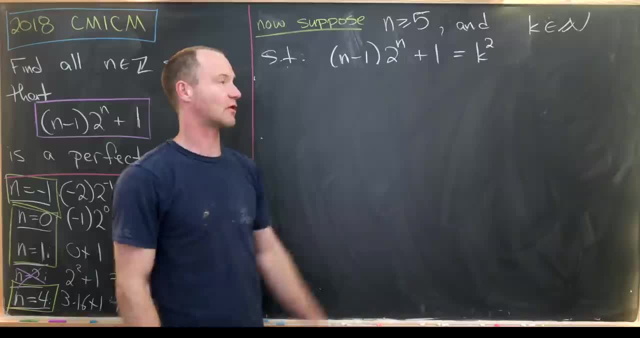 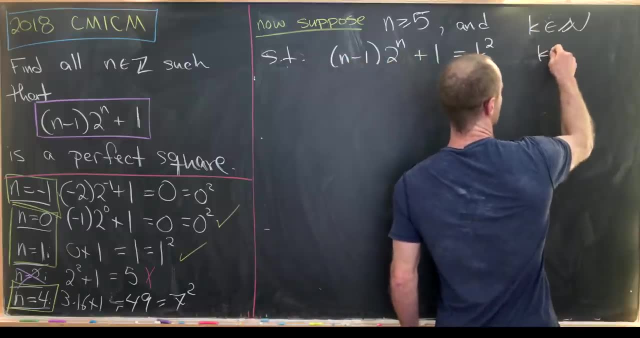 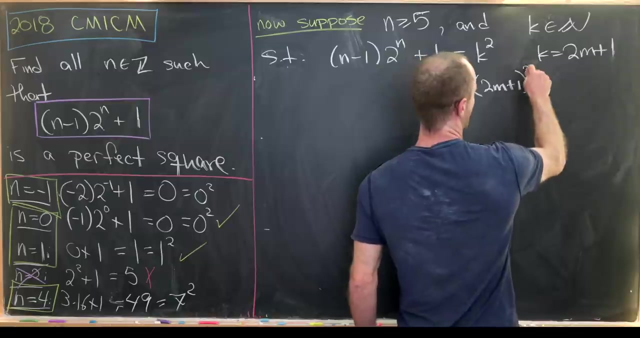 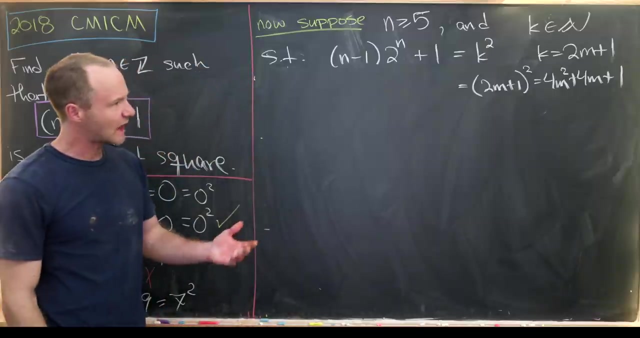 definitely an odd number. That's because this bit is even and we're adding 1, so that means that k is an odd number. But since k is an odd number, we can write it as 2 times m plus 1, which means this is 4m squared plus 4m plus 1.. Now we can start to simplify a little bit. Notice that we can. 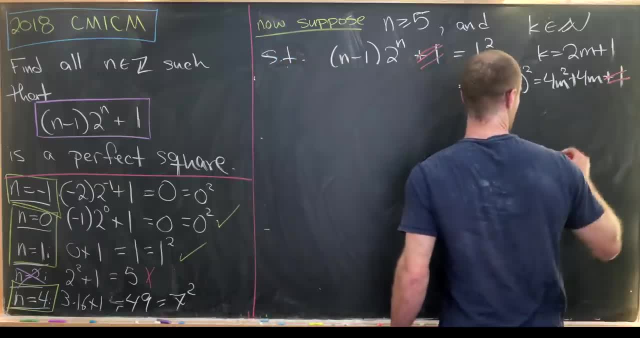 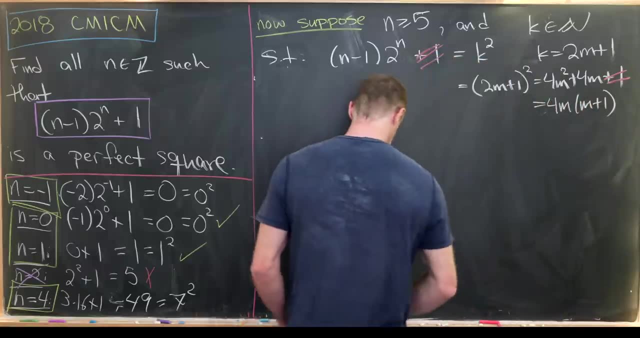 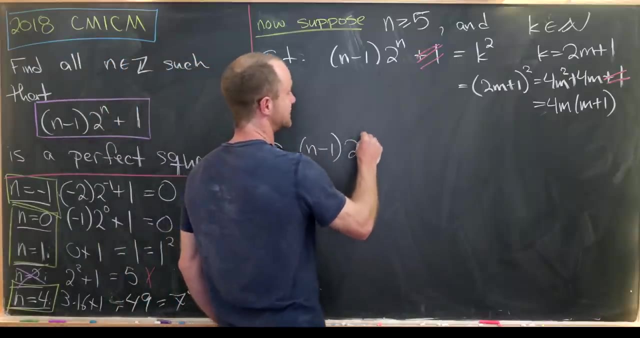 subtract 1 from both sides of this, and then we can also factor a 4m out. That leaves us with 4m times m plus 1.. Then we can divide both sides by 4, leaving us with the equation n minus 1 times 2. 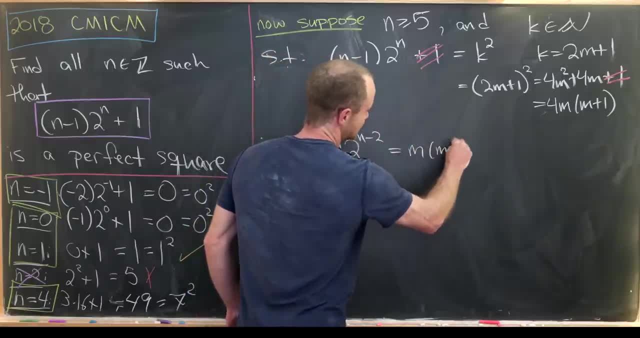 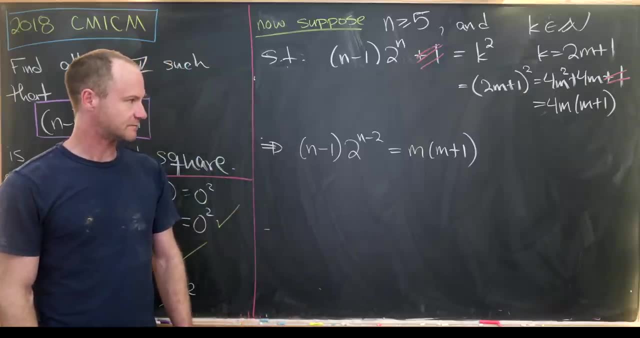 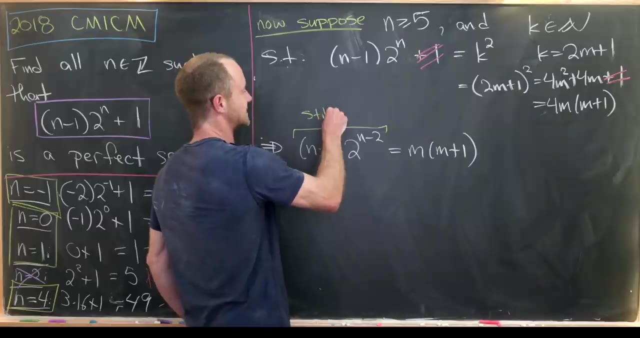 to the n minus 2 equals m. Okay, so that's starting to shape up quite nicely. Now let's note that the left hand side is still even. We know that this left hand side is most definitely still even because we know that n is. 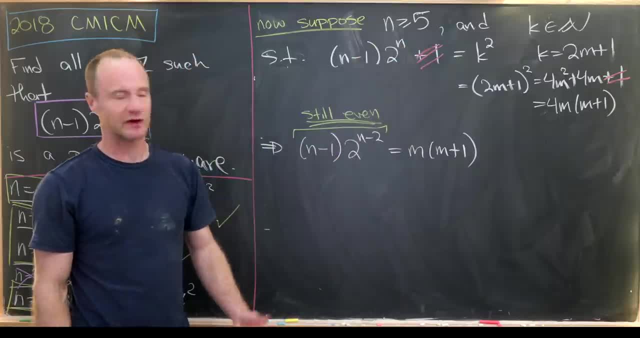 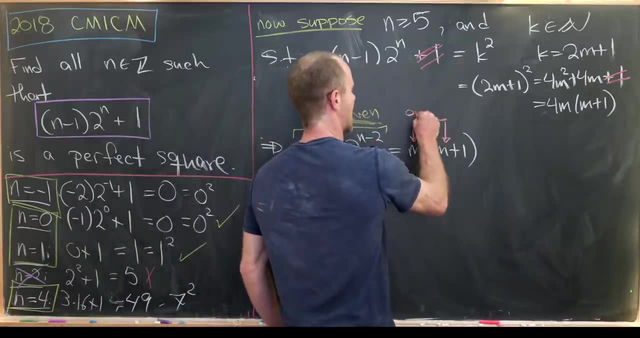 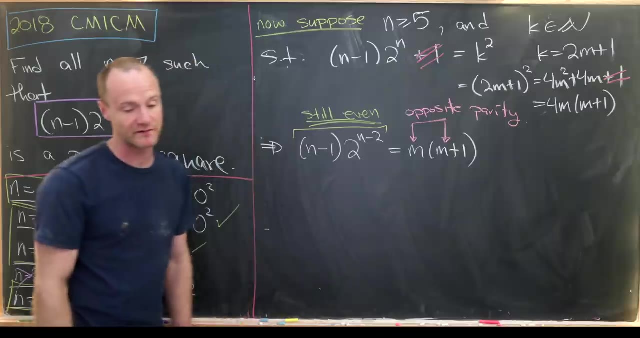 bigger than or equal to 5, so that this exponent here is bigger than or equal to 3.. Another thing that we know is that these numbers right here, m and n plus 1, are equal to 3.. So we know that m plus 1 have so-called opposite parity. So when I say they have opposite parity, that means one of 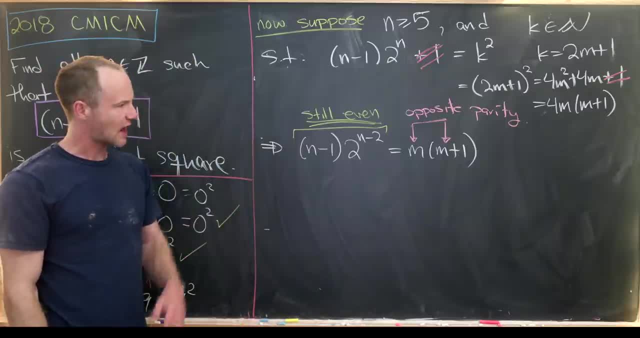 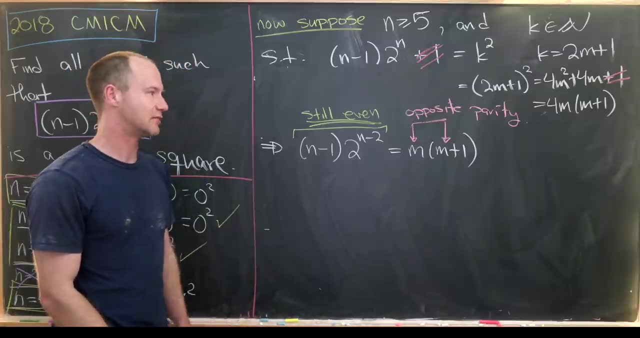 them is even and one of them is odd, And so now we'll just like work through both cases. What if the case is m is even? or what if the case is m plus 1 is even? So let's take that first case first. 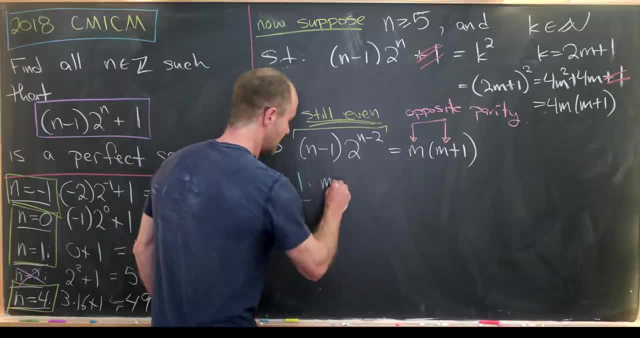 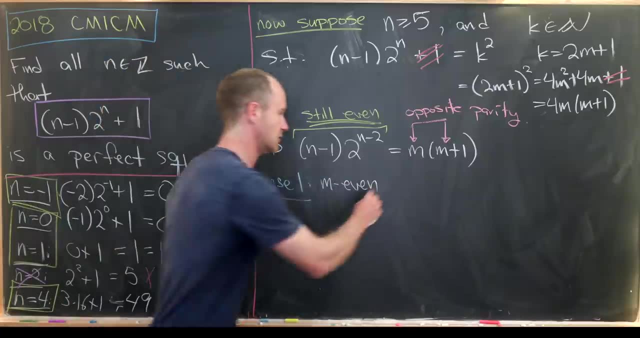 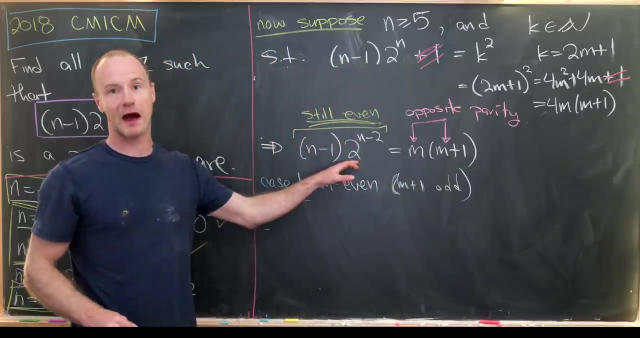 So case number one: m is even. Okay, so since m is even and m plus 1 is odd, Well, let's maybe put that down: m plus 1 odd, That means that m gobbles up all of the powers of 2 here, Because if it didn't gobble up all of the powers of 2, then 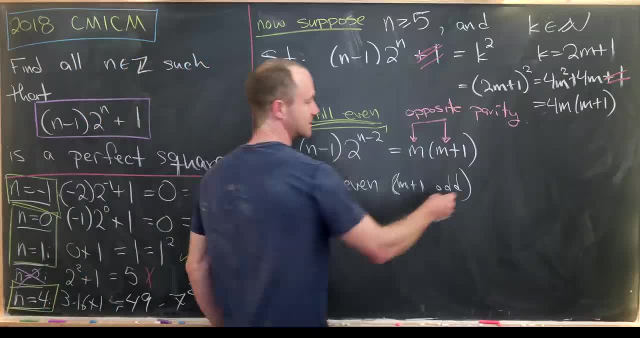 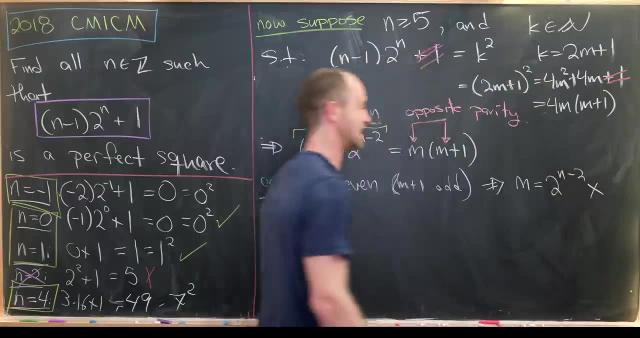 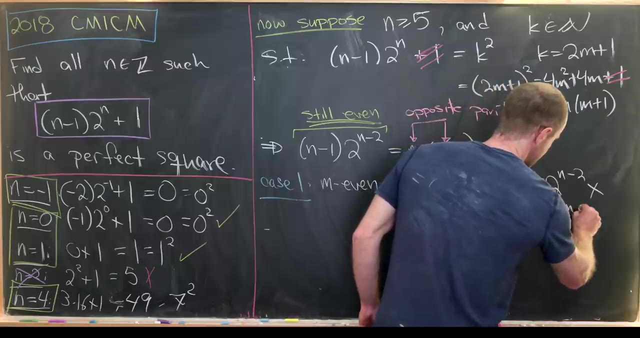 m plus 1 would also be even, which is a clear contradiction. So that means we can write m as 2 to the n minus 2 times x. Okay, and then from there we can write m plus 1 as 2 to the n minus 2 times x plus 1.. Because it's clearly just equal to m plus 1.. 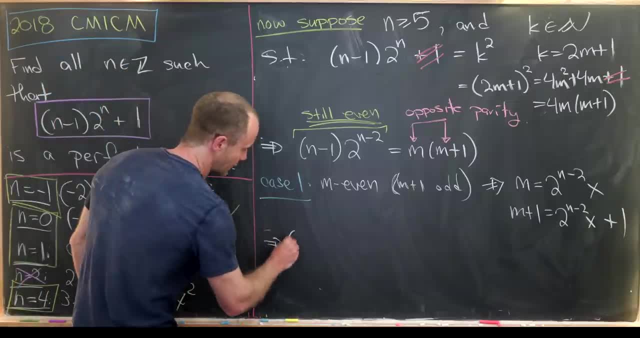 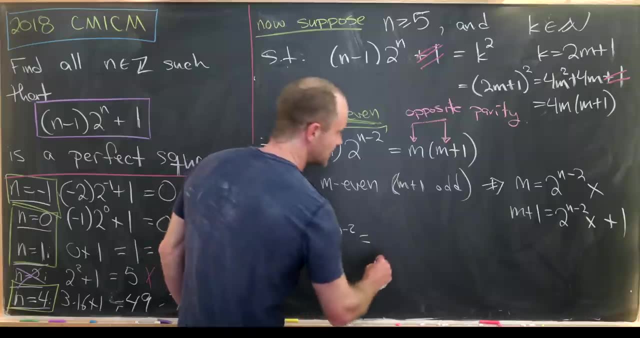 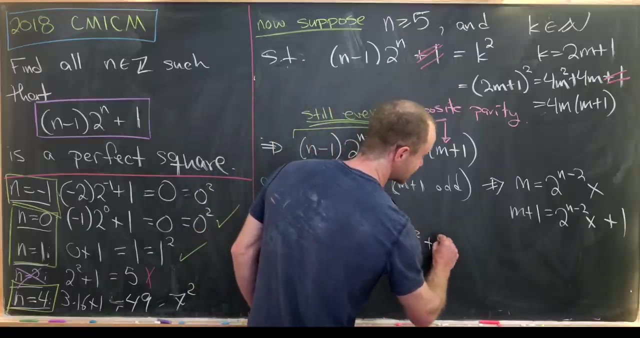 Okay now where does that leave our equation? We have n minus 1 times 2 to the n minus 2 is equal to: let's see: we have 4 to the n minus 2 times x, squared plus 2 to the n minus 2 times x. 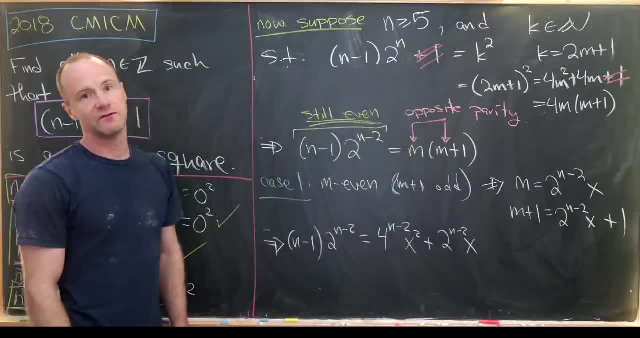 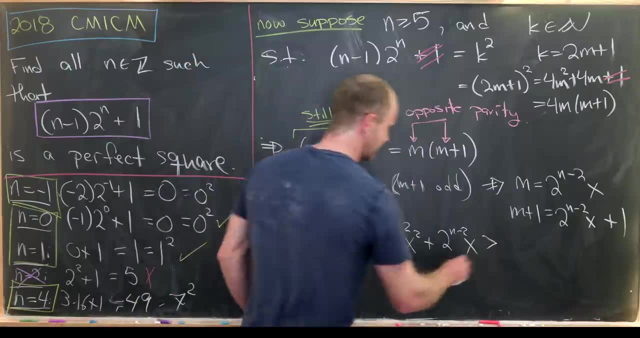 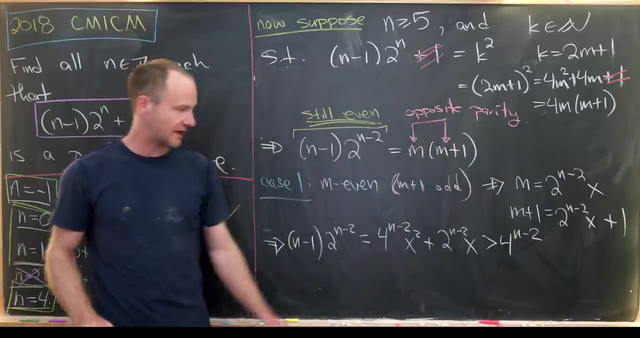 So that's just from multiplying this thing through, given those values of m and m plus 1.. But now we're going to work towards another size contradiction. So let's note that this is most definitely bigger than 4 to the n minus 2.. And that's because x is bigger than or equal to 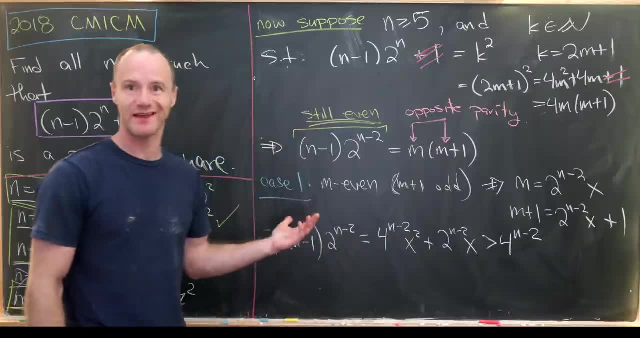 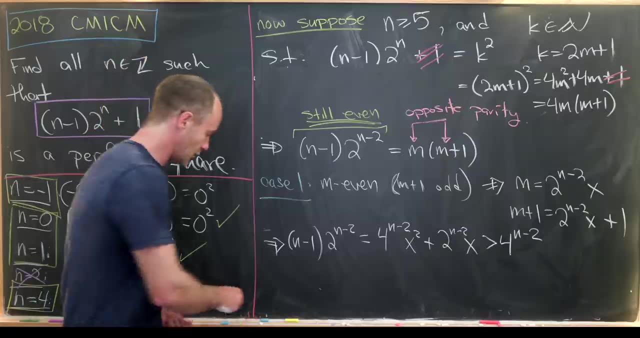 1 here, So we can get rid of this guy right here and then just maybe, like, get rid of the x term, keeping in mind that multiplying by x squared will give us something larger. Now we'll take what's left over, which is this inequality right here, and divide both sides by 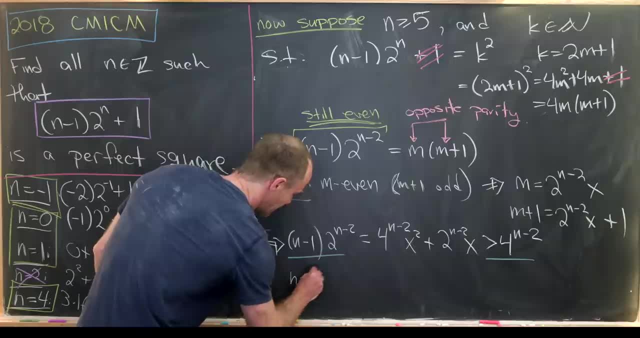 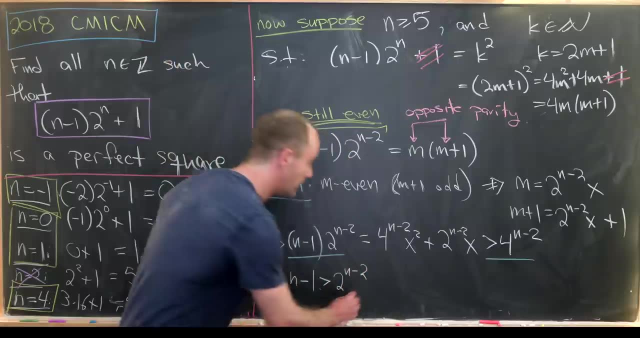 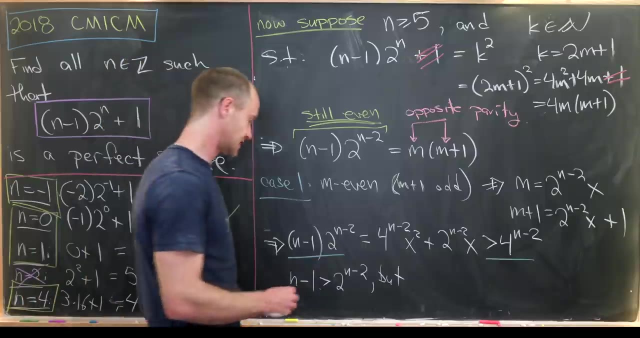 2 to the n minus 2, leaving us with n minus 1, is strictly bigger than 2 to the n minus 2.. But we could prove- maybe a version of what we just did for that last case, that negative case, to show that 2 to the n minus 2 is. 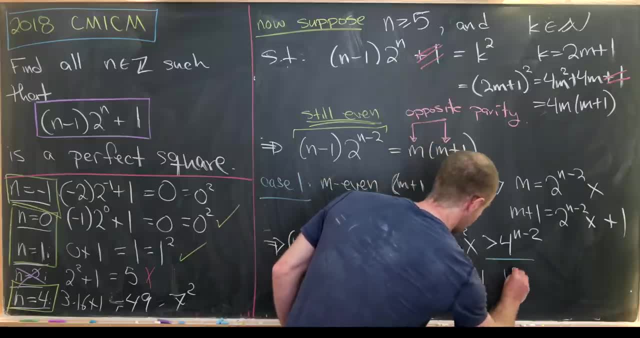 bigger than n minus 2.. So we can get rid of this guy right here and then just maybe like get rid of this guy right here and then just maybe like get rid of 2 to the n minus 1 for all n bigger than or equal to 5.. 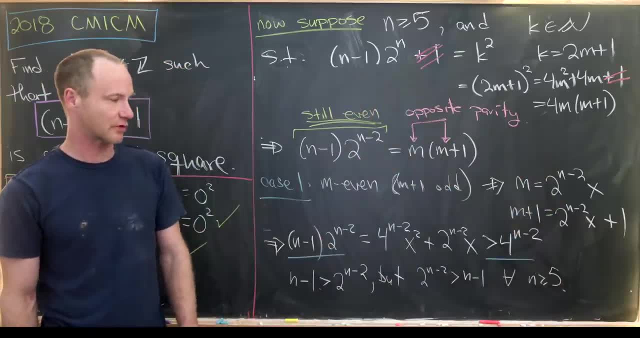 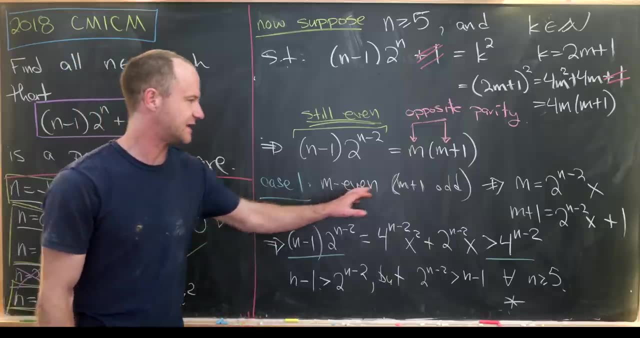 So I won't do that here, because that's essentially the exact same proof that we did for that previous case. So that brings us to a contradiction. So now let's move on to the second case, where we have these parities switched. Now we're ready to finish this thing off with the case where m plus 1 is. 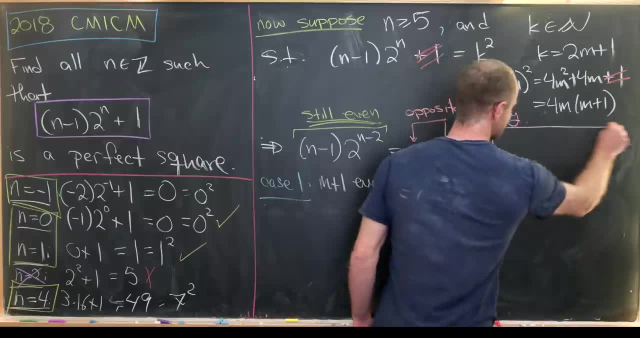 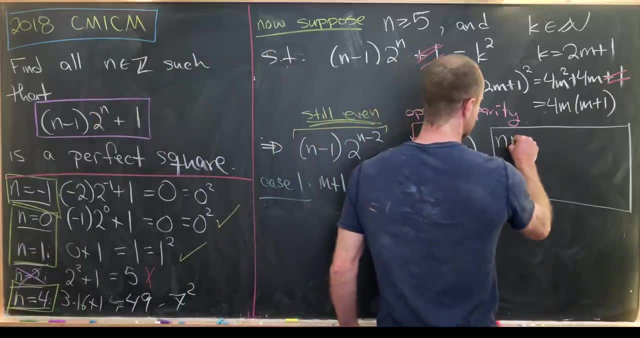 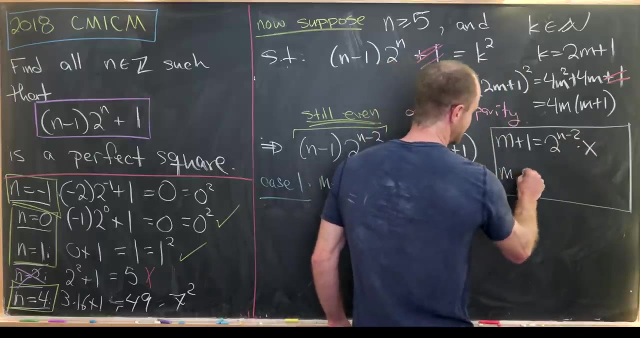 even and m is odd. That gives us the same type of decomposition as we had before. We know that m plus 1 has to gobble up all of the powers of 2.. So we have m plus 1 is equal to 2, to the n minus 2 times an integer x, which means m. 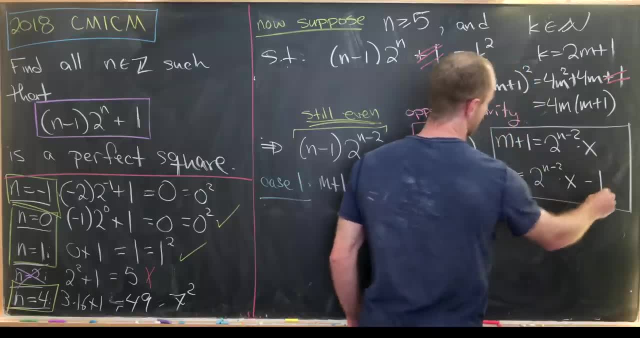 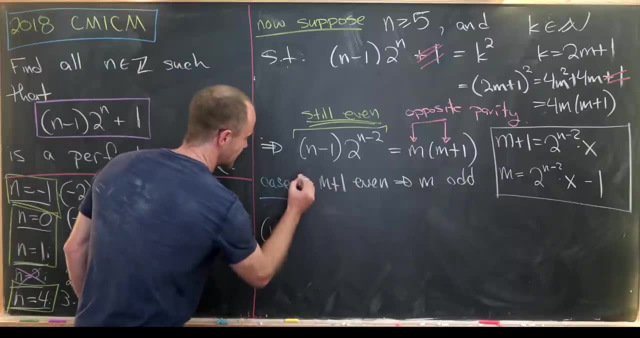 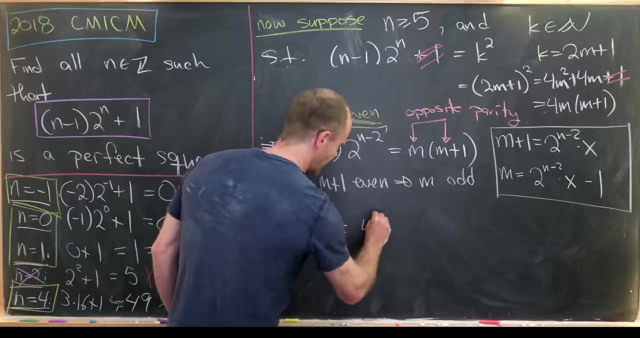 is equal to 2 to the n minus 2 times that integer x minus 1.. Okay, but now plugging that into this equation right here gives us n minus 1 times 2 to the n minus 2 equals. let's see, we'll have 4 to the n minus 2 times x, squared minus 2 to 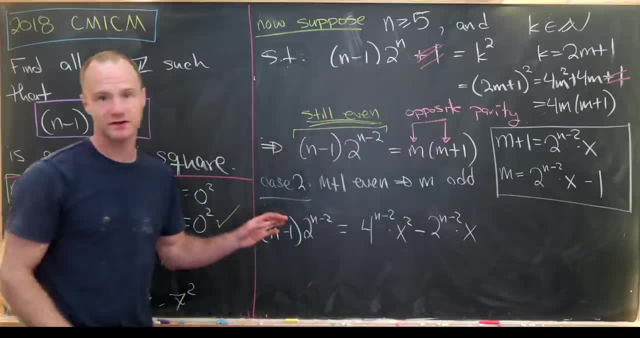 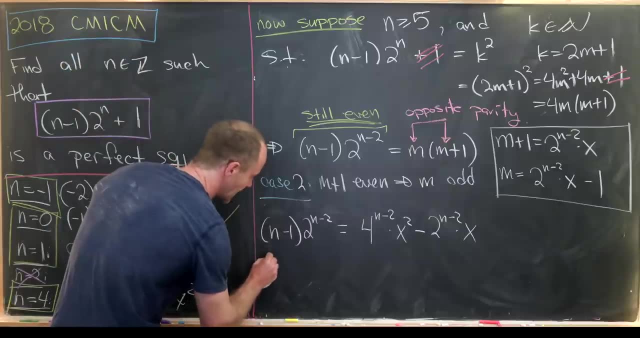 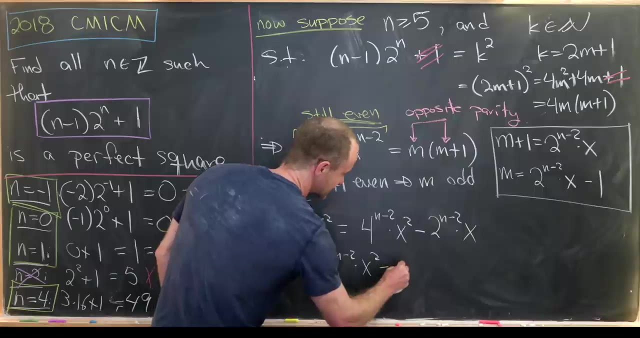 the n minus 2 times x. So something that looks like that: Now, from here we'll divide both sides by 2 to the n minus 2, and that'll leave us with n minus 1 equals 2 to the n minus 2 times x, squared minus x. 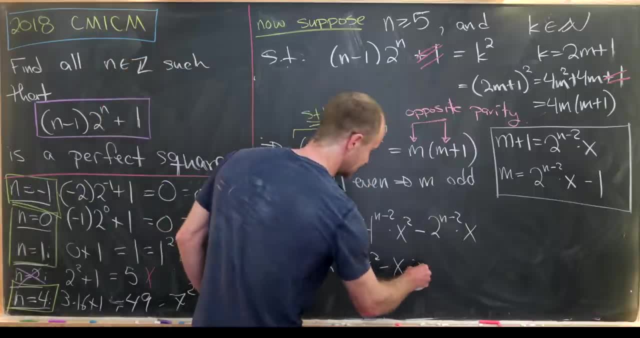 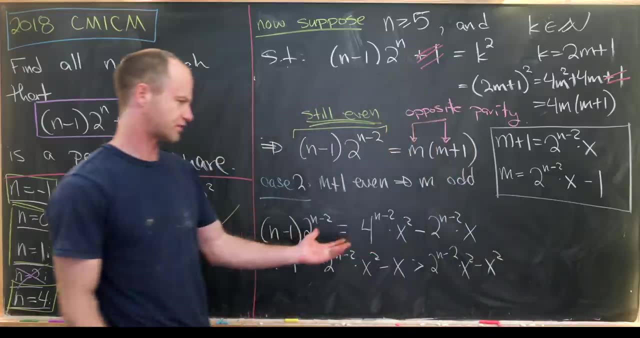 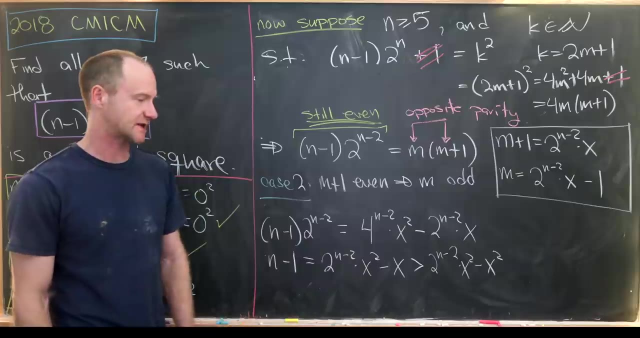 But now, since x is a natural number, we know that this thing is bigger than 2 to the n minus 2 times x squared minus x squared. We just replaced x with x squared, creating something smaller, since we're subtracting it. 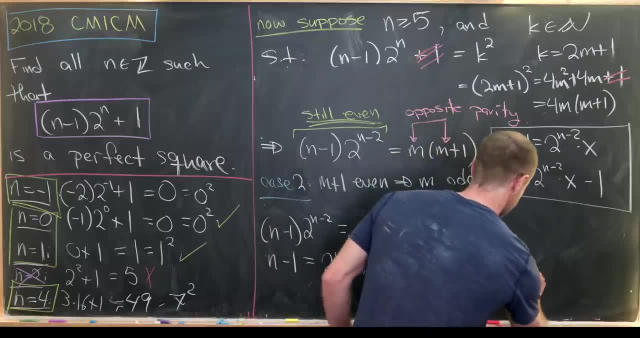 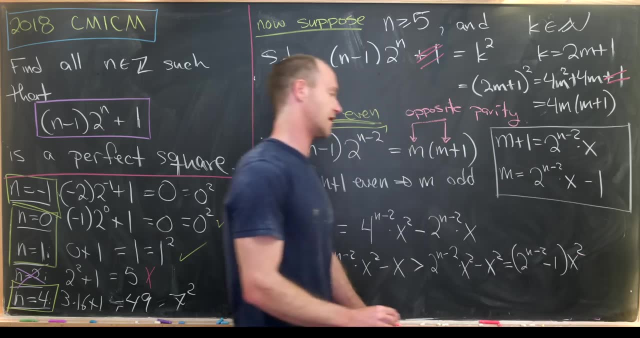 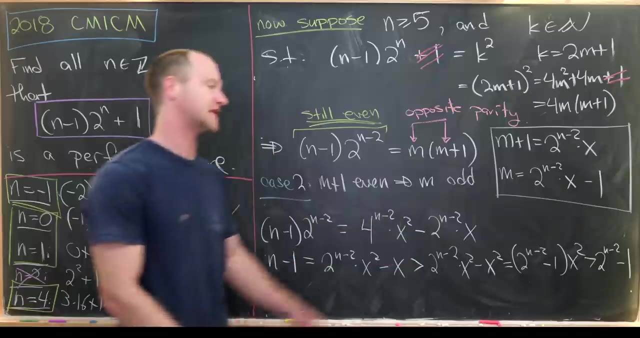 Now we can factor an x squared out and notice that that gives us 2 to the n minus 2 minus 1 times x squared. But now that itself is bigger than 2 to the n minus 2 minus 1, again because x is bigger. 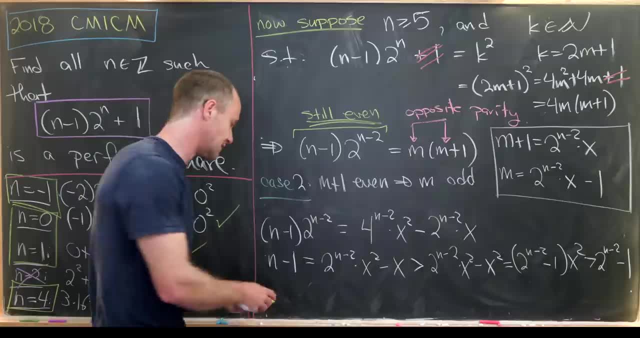 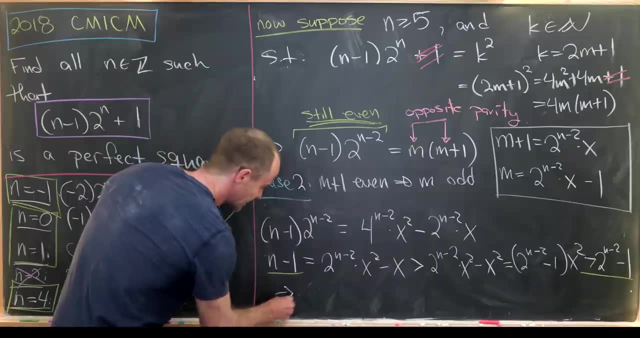 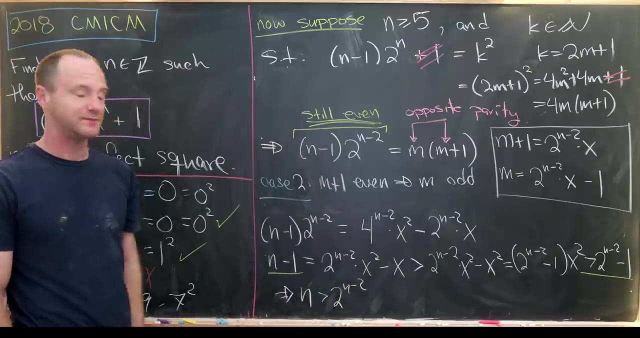 than or equal to 1.. Okay, so now let's see what we have here. We have: n minus 1 is bigger than 2 to the n minus 2 minus 1,, which tells us that n is bigger than 2 to the n minus 2,, which means that n is bigger than 2 to the n minus 2,. 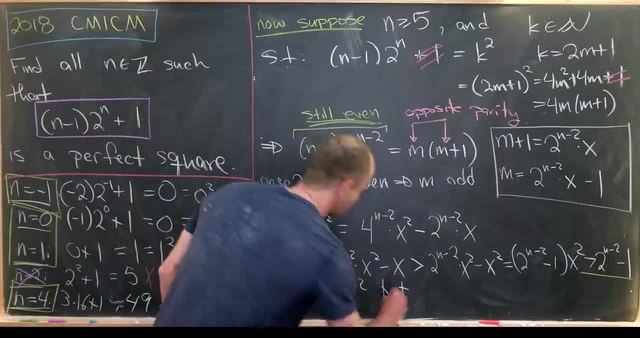 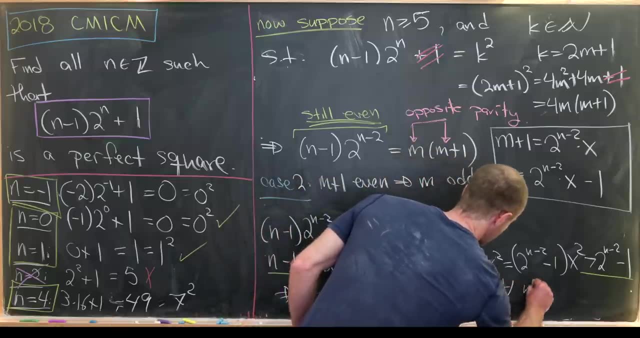 which again will give us the same solution. So that's sort of inequality type of contradiction as we had before, because n is less than 2 to the n minus 2 for all n bigger than or equal to 5.. Again, you can check that, just as we did for those other cases.